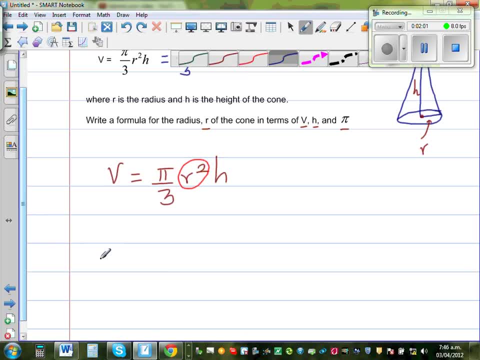 blue color. so if I want to get rid of this pi over 3, what's the op? how will you cancel pi over 3? so well, the op, I want to. if I want to cancel this pi over 3, I have to multiply this side by 3 over pi, because the opposite of pi over 3 is: 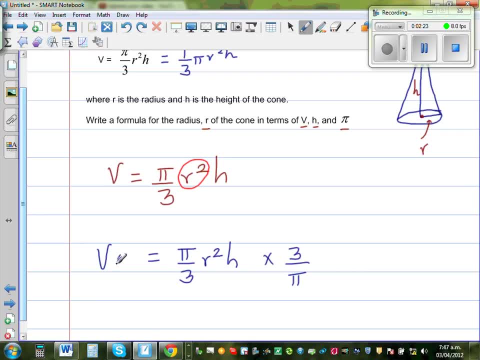 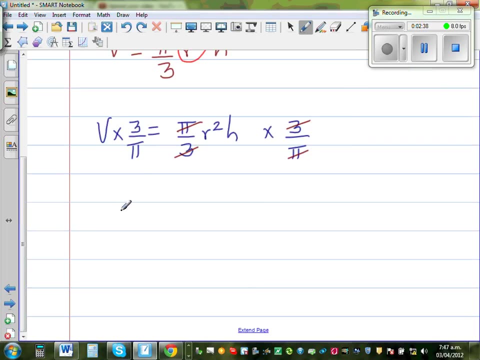 3 over pi. so if you multiply this side by 3 over pi, I'd also multiply this side by 3 over pi. so what'll happen? so 3 & 3 gets canceled, PI & PI gets cancelled. so we have done one step at the time. so we can say: well, so this is 3b over pi now. 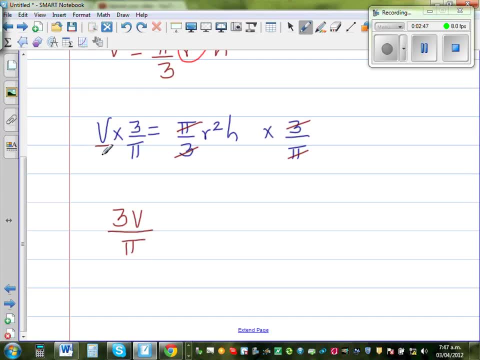 you may want to write down the y series in the estándar if you check out the company to jumf. so you may want to write down the y series in the estándar. if you check out the company to jumf, the value to get a 3v v has a denominator of 1, so basically you're multiplying v times 3 is 3v. 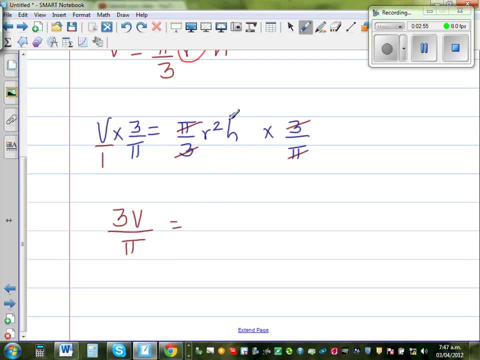 and 1 times pi is pi is equal to what is left over r squared h. okay, so now what should i do? i want to get rid of this h from this side, so i'm going to divide this side by. i'm going to divide this side by v. sorry h. i'm going to divide this side by h. 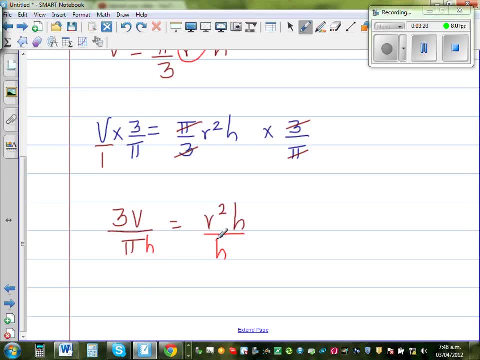 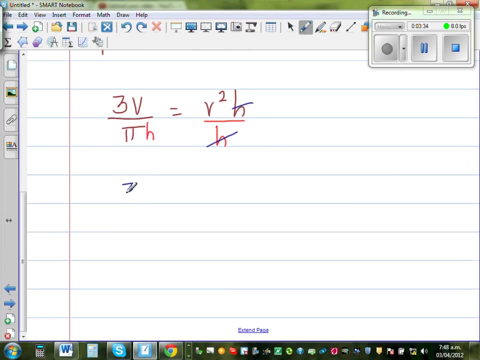 so i can also divide this side by h, just like that. so this: i'm putting a denom h in the denominator here, so to put it down h in the denominator, so i'm dividing both sides by h. so what happens? h and h gets cancelled. okay, so now i can write 3v over pi h. 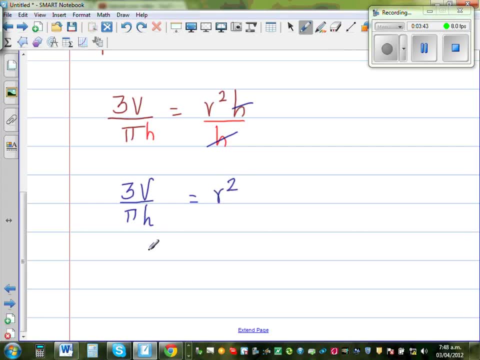 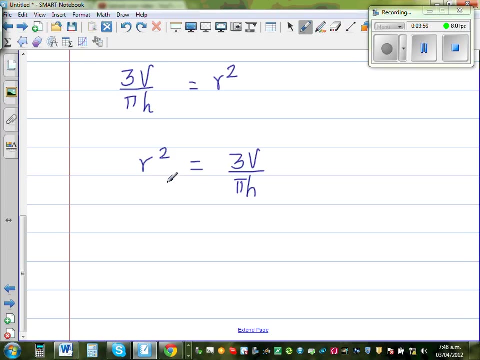 is equal to r squared. so let me write the other way around, so i can just say: r squared is equal to 3v over pi h. okay, so now, if i want to get rid of this r squared, what should i do? what's the opposite of r? squared or squared? what's the opposite of r squared, sorry, squared? 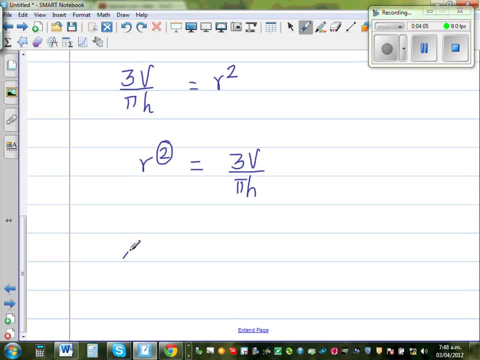 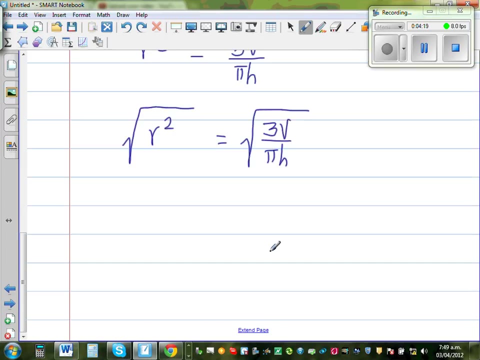 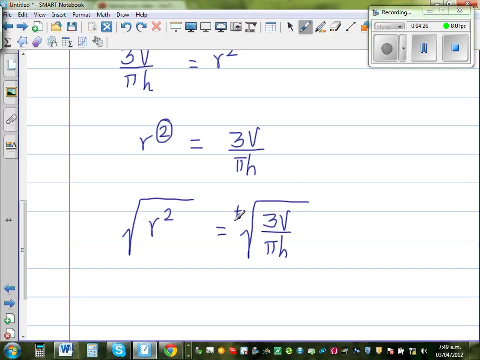 the opposite of r squared is square root. so to take the square root of this side, so square root of r squared is equal to square root of 3v over pi h. so whenever you do square root of, uh, square root of the right hand side here, to put plus or minus, here i'll explain why. 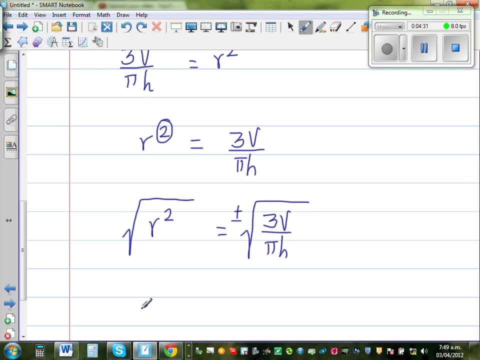 so yeah, so square root of r squared is: r is equal to plus or minus square root of 3v over pi h. now why? why should we put plus or minus? i'll explain that suppose. let me do a side example here. okay, suppose you have x: squared is equal to say 36.. 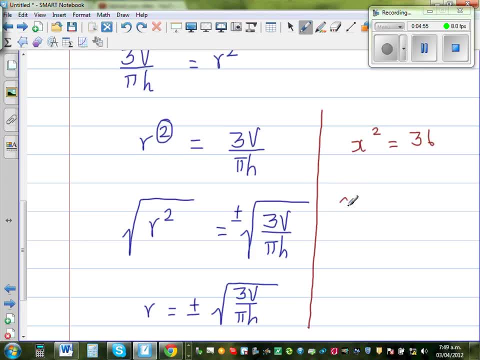 i want to get rid of this square. so what should i do? i should do square root of 30, sorry, square root of x squared. square root of x squared is equal to- i should put plus or minus- square root of 36. i'll explain that here. 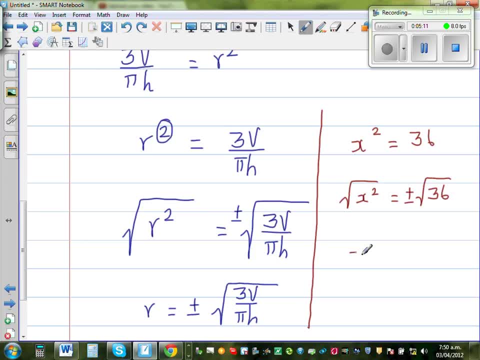 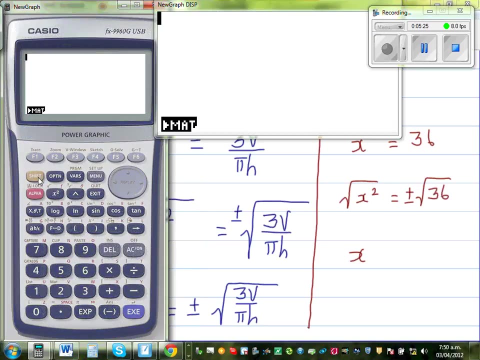 y and square root of x squared is x. okay, some of you may wonder how did they get this? so square and square root are opposite of each other. okay, so let me show that on the calculator. so if you go to run- suppose if you go shift, square root of phi squared. 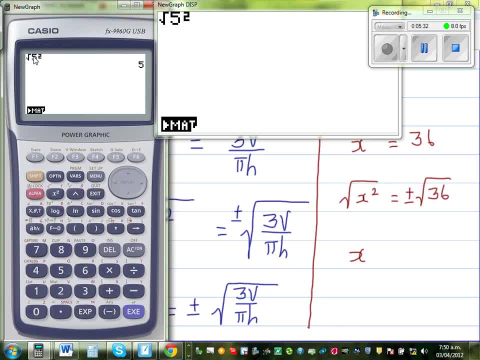 is phi okay. so square and square root cancel each other out. square root of- sorry shift. square root of, say, 100 squared would be 100. so square and square root cancel each other out. so you get 100. but when you're finding square root of a number you have to put plus or minus. 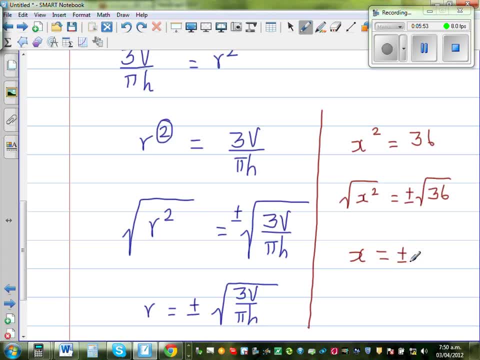 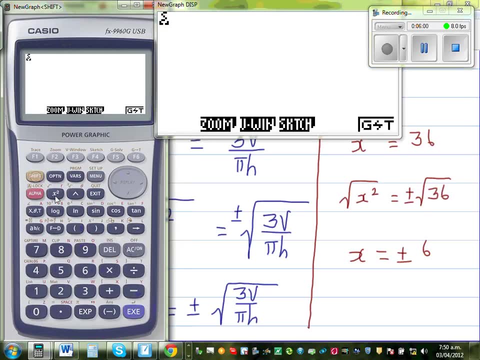 i'll explain that too. so this is nothing but plus or minus. square root of 36- i hope you know- is 6.. on a calculator, it will give you only one answer. if you do square root of 36, it will give you only one answer. by default, it's only giving you a positive answer now.